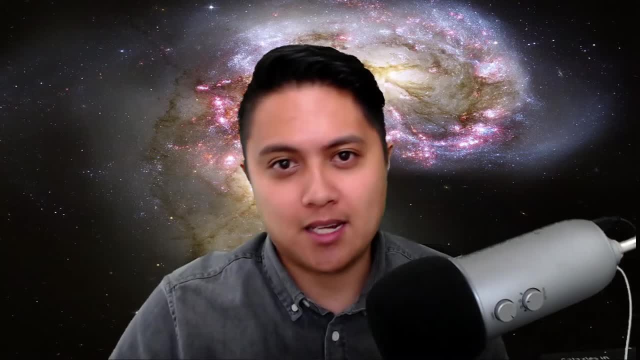 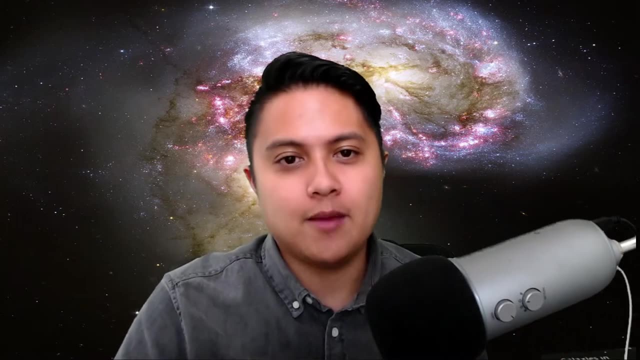 getting a little bit out of date. Binney and Tremaine came out in 2008 and Binney and Merrifield came out in 1998.. So they are on the older side And it just seemed time for a new book to come. 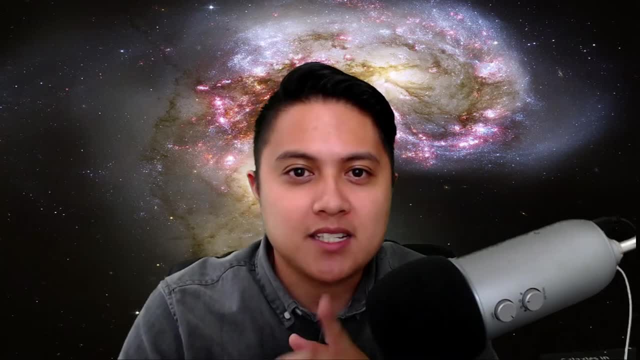 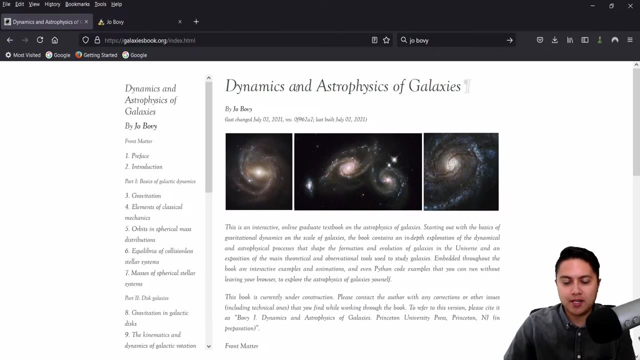 about, And I'm happy to announce that that is exactly what I'm going to be doing. I'm going to be doing a lot of research on this, So I'm going to go here to my web page browser. We can see here this online textbook: Dynamics and Astrophysics of Galaxies by Joe Bovee. Now, for those of you, 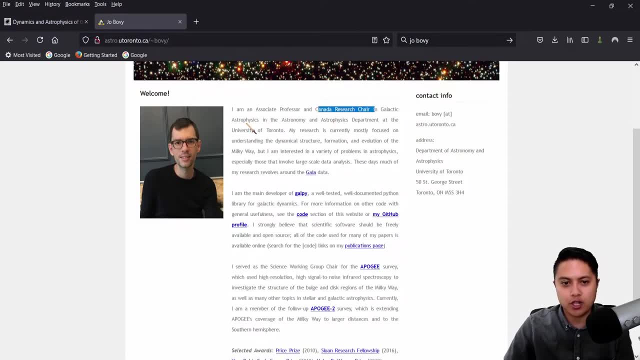 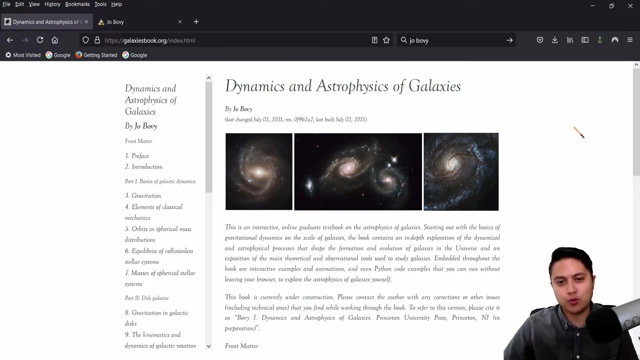 who don't know. Joe Bovee is the Canada Research Chair in Galactic Astrophysics at the University of Toronto And he is the main developer of GalPi, which is this documented Python library for Galactic Dynamics. I've used it a few times in my own research. It's super, super useful And 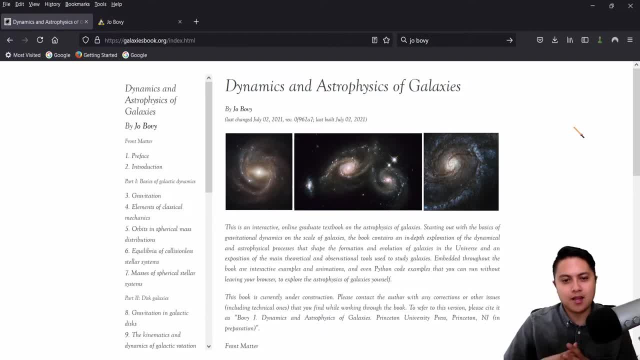 he is making this online textbook that is interactive, where we can read about the theory- sort of the same sort of material that we see in Binney and Merrifield and Binney and Tremaine- but we'll also have online interactive examples to help drive the points home. So I'm going to 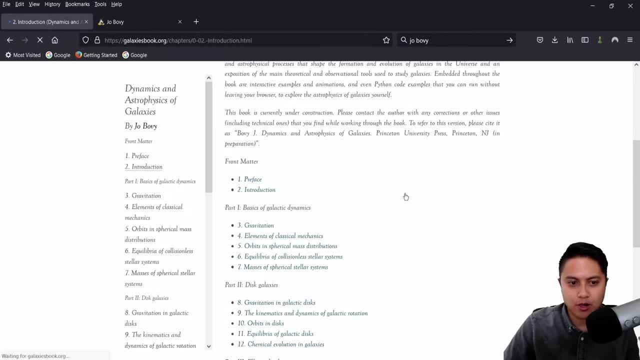 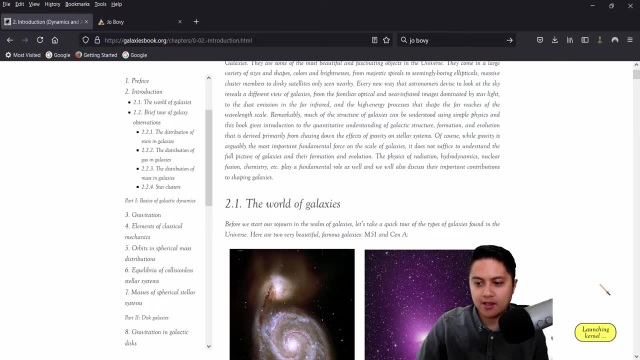 actually click on a chapter here. Let's go like introduction, for example, And I'm going to move myself so you can see this, But you can see here that there is this make interactive button and then if you click, I believe we'll launch the different Python kernels that we can run code on. 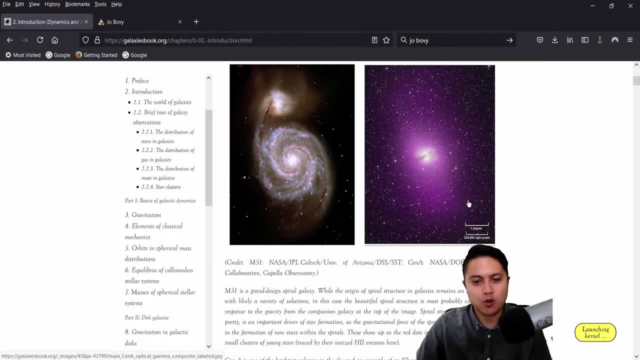 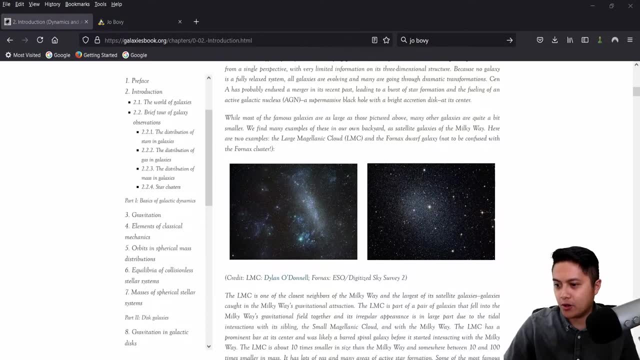 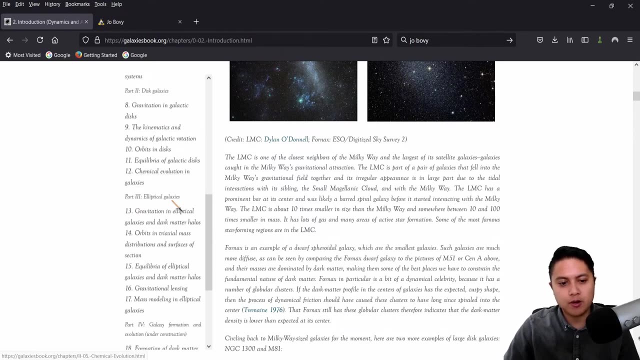 And so we can understand the physics that's going on, but also see it applied in this Python code. So I'm going to move myself back now because I'm watching the kernel. It'll tell me when it's done. And you can also take a look at the different contents of the book right here. The first three: 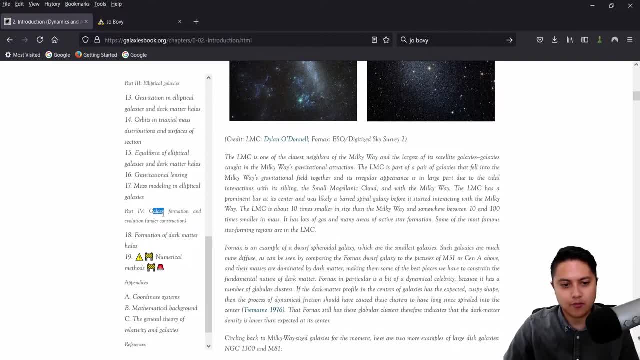 parts I believe are done. He hasn't finished the fourth part, which is Galaxy Formation Evolution, which includes formation of Dark Man and Halos. And then we'll move on to the next part, which is the Galaxy Formation Evolution, which includes formation of Dark Man and Halos. numerical methods. 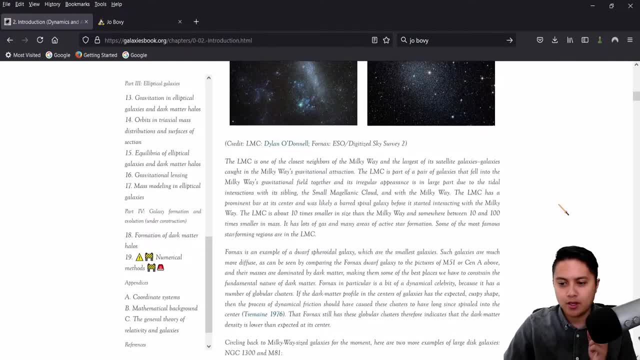 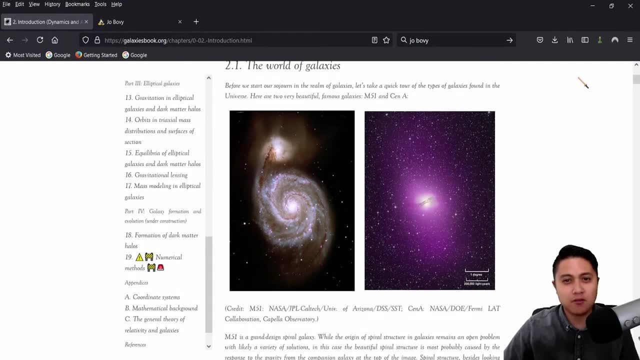 which is all very, very relevant to research today. But I'm just super stoked for a book like this to come out. because I'm still in grad school, You know this is still going to be super useful. Dynamics is a very, very big and interesting topic that I think would mesh well with my 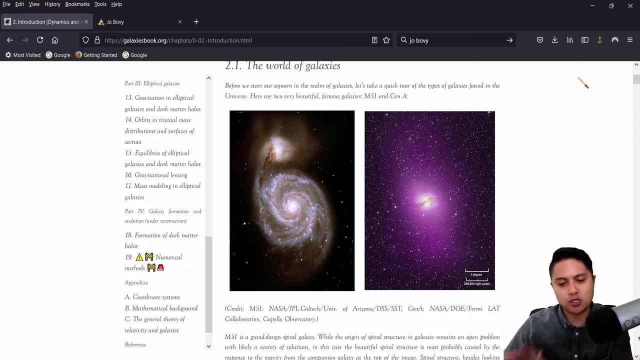 research because since I do gas dynamics, I focus more on the gas as opposed to the stars. but gas and star-based black hole mass measurements have shown to disagree over time And I think getting to know more of the stellar dynamics slash galactic dynamics. 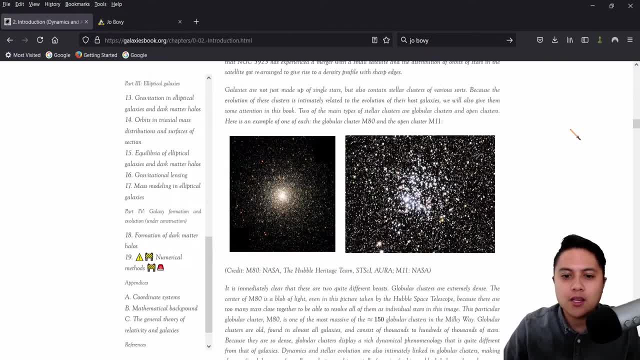 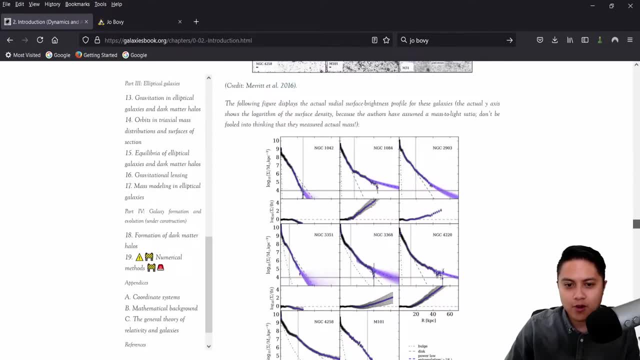 methods is incredibly important in my own development as a scientist, And so I'm just absolutely stoked to see a book like this hit the market. And from what I can tell so far, I mean the pictures look great. I haven't seen any kernels yet, but it looks. Oh, 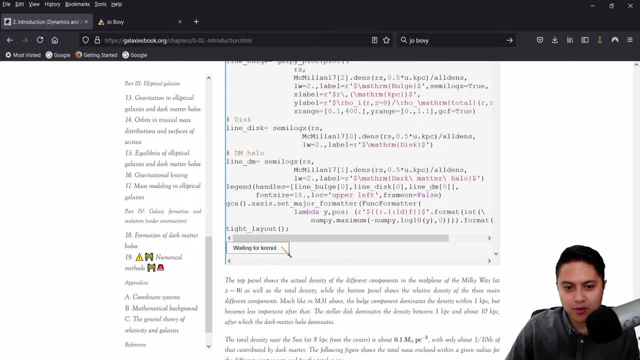 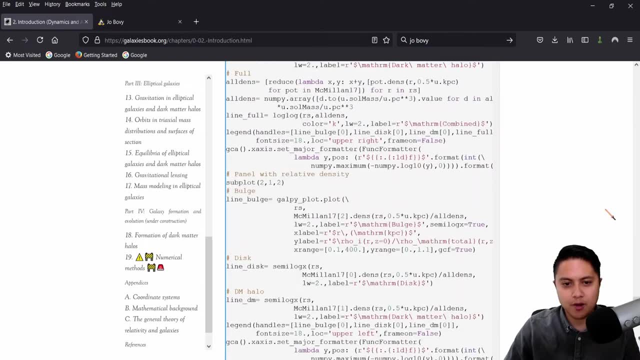 here's some kernels, So here's some Python code that we're still waiting on. Apparently, it takes a while to load, But I am really hyped because, to be honest, both those books- Binney and Merrifield and Binney and Tremaine- they're very dense and they're 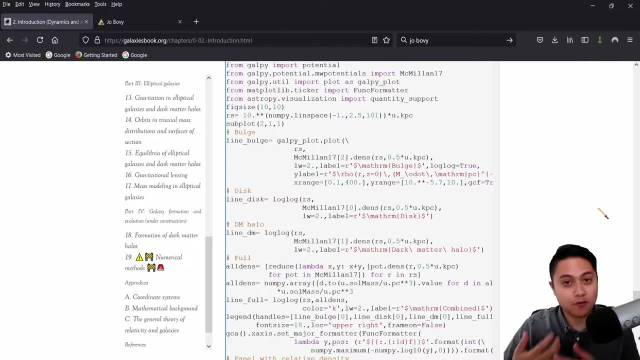 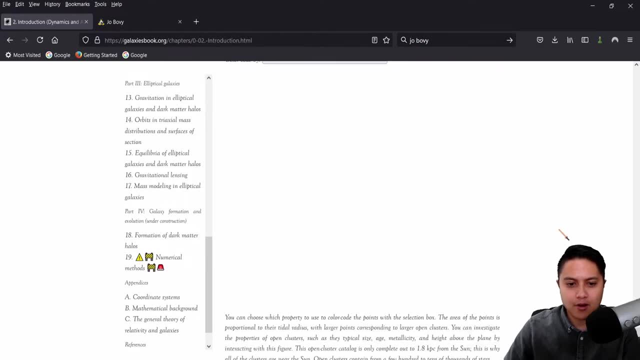 quite difficult to wrap your head around and really learn from, because they're more of reference books as opposed to textbooks, that you try and learn something for the first time, And so I'm very, very happy to see a book like this hit the market. Looks like it's taking a 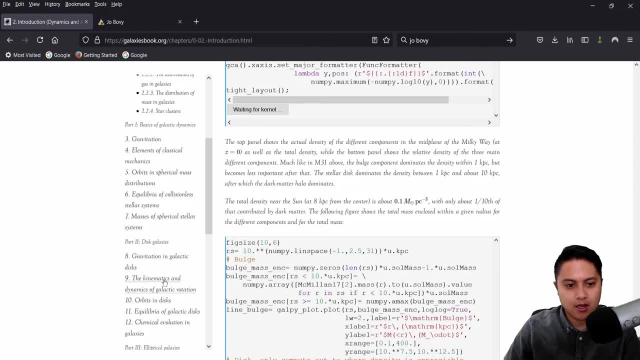 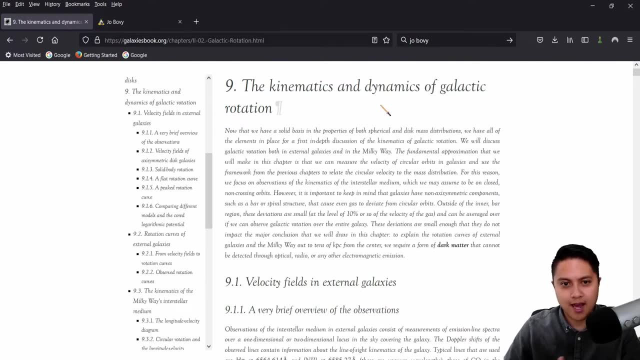 while for some of this stuff to load. So I'm just going to go ahead and pick a different chapter. Let's do chapter nine: the kinematics and dynamics of galactic rotation. My research is more small scale rotating gas discs, So while these are on the scales of entire galaxies I'm usually looking at 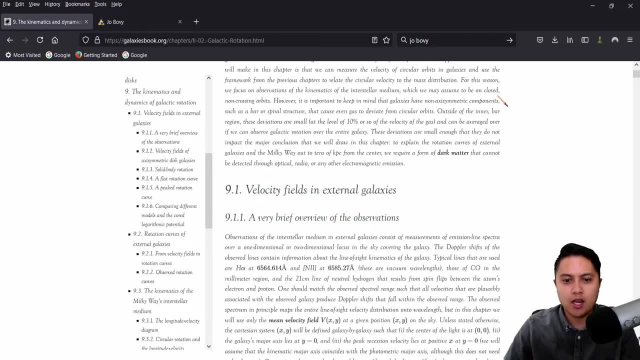 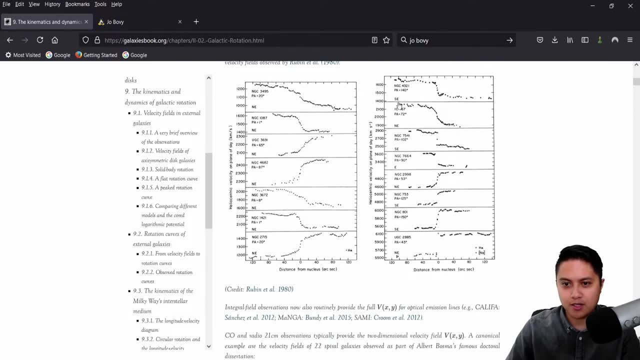 gas discs that are rotating very close to the center of the galaxy in orbit around a super massive black hole. But all of this stuff is actually very, very, very related to what I do in my own research. I mean, this is a rotation curve. I generate plots like this in my own. 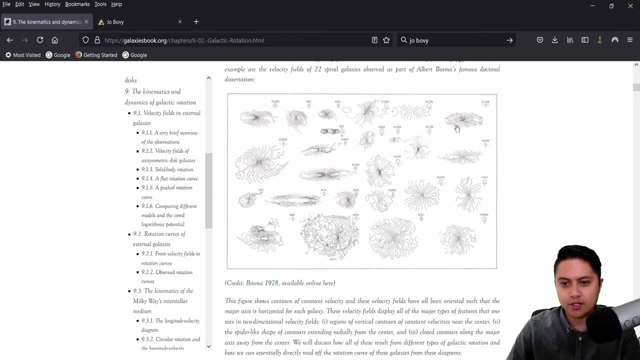 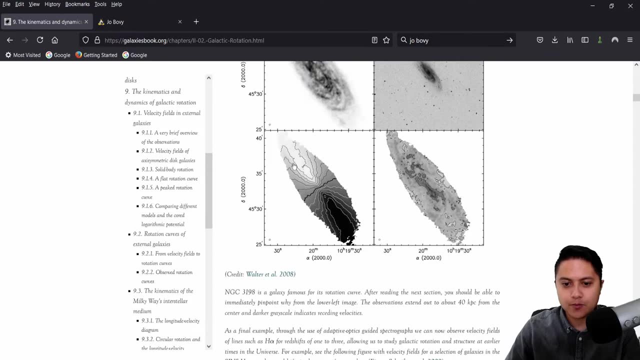 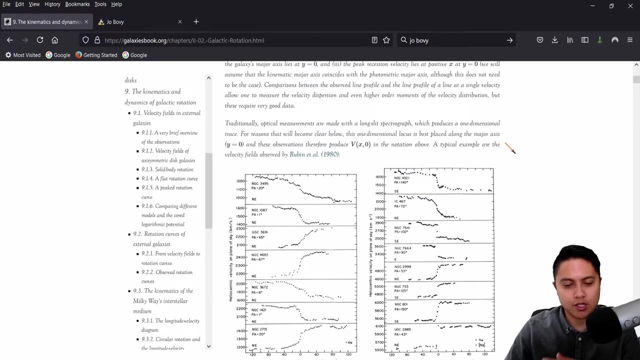 research. These are sort of spider diagrams showing the velocity fields of rotating disc galaxies And again, this is all stuff that is pertinent to what I do. So if you're very interested in my own research and sort of what goes into breaking the stuff down and knowing what's going on, I think this chapter will be very 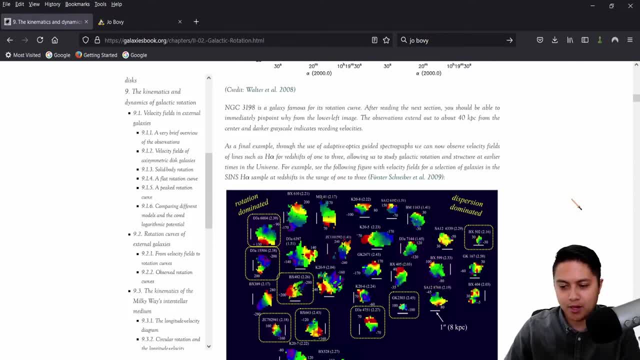 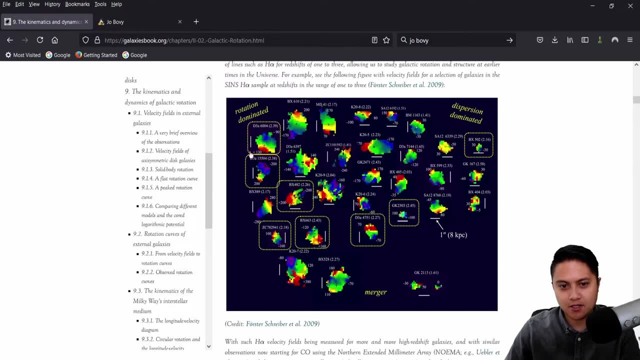 very helpful for that purpose. I'm going to click the make interactive button on the bottom corner here and we're going to take a look at some of the kernels. So here these are what H alpha velocity fields which show the um, the velocities of the H, of the H alpha emission across the 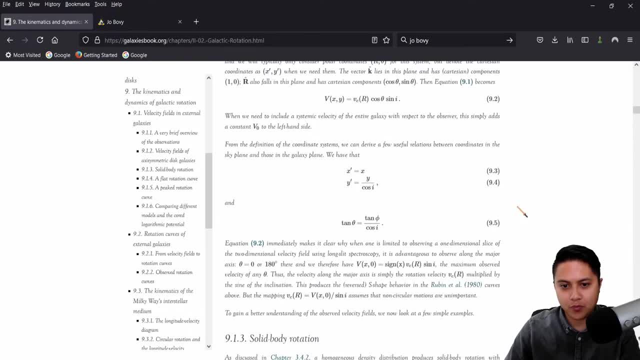 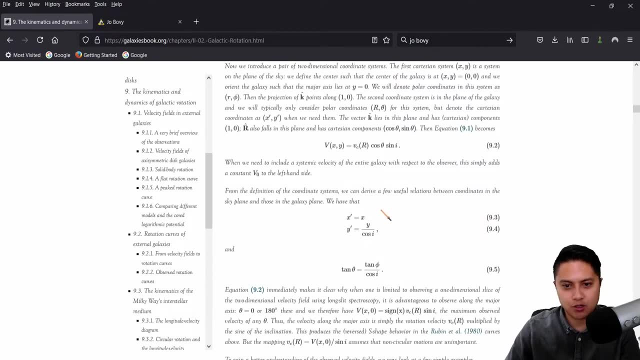 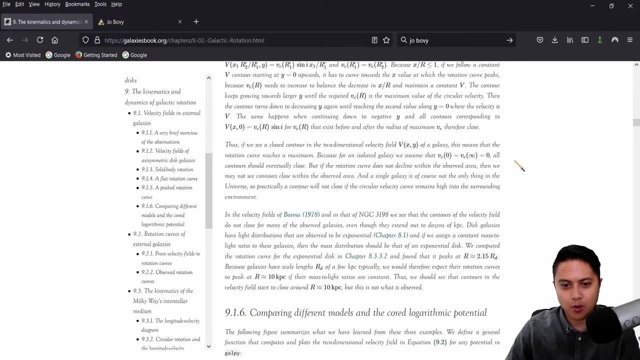 different discs here. And um, oh th. this is um. this is oh yeah, velocity fields of asymmetric disc galaxies. Again, this has actually been transformed into code in my own research, So I I use these formulas in my own research. It's really cool to see this all broken down and have 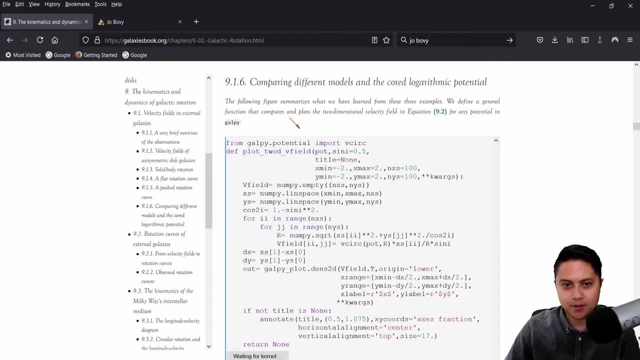 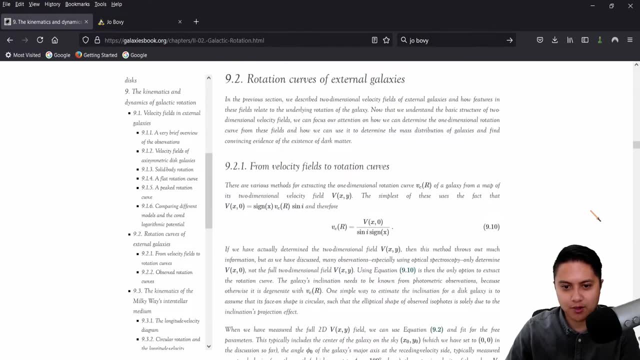 all these different examples And, um, here is, uh, a kernel- Python kernel- that I'm waiting for And I'm still waiting for. I think I'll just scroll down and just read a little bit more, But I'm not going to go through this whole book just because it would take too long. 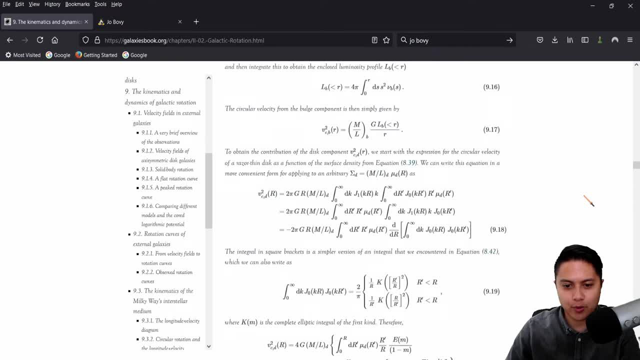 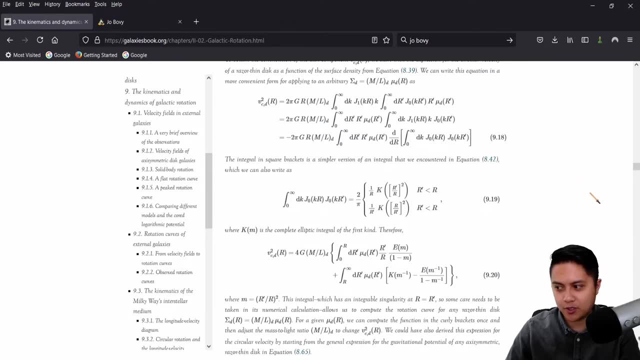 but I think it's. it's super awesome to see a book like this just coming out soon And I definitely I think we'll get a physical copy when it's when it's released, because this is. I'm getting excited just reading this. I don't know if you can. 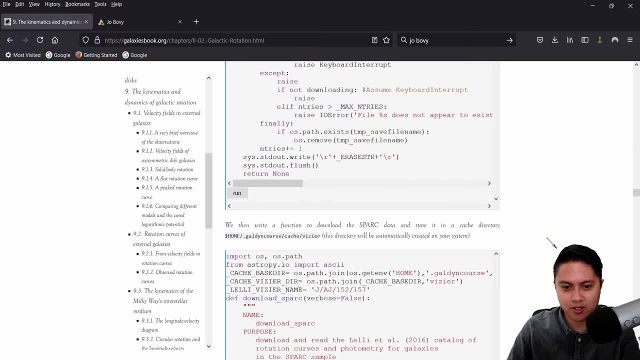 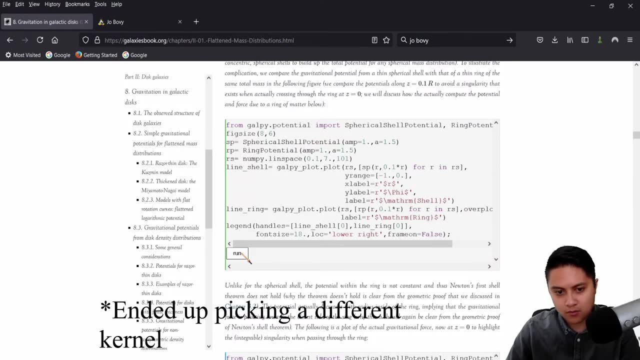 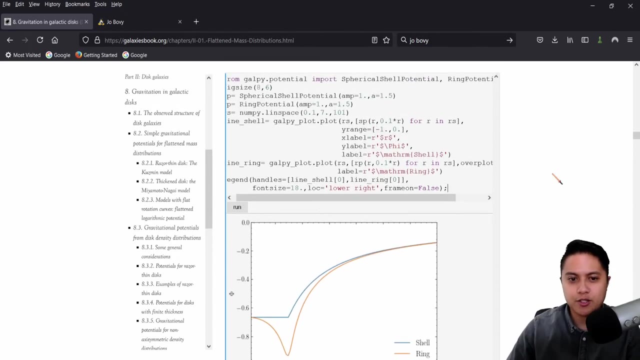 tell that I'm. I'm getting so hyped looking at this, So it looks like the kernel is loaded, So I'm going to go ahead and hit, hit, run here, So I think we'll have to wait a little bit. Aha, Okay, So I just ran a different cell in chapter eight and 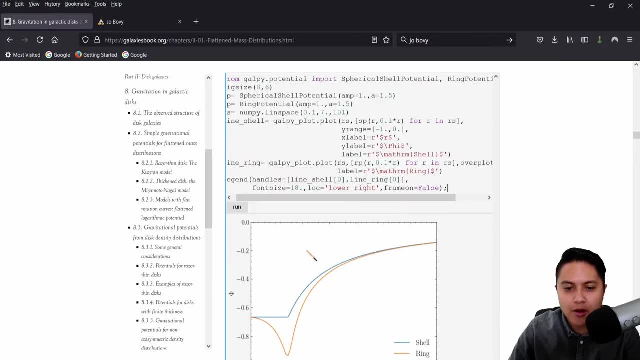 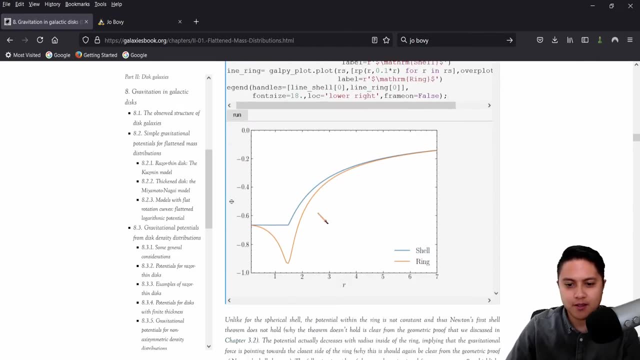 what it produced was this plot. I guess it's comparing a shell versus a ring for for a mass distribution, And this is just super cool. I mean this is just. I mean I wish all textbooks could be like this, that this is the direction that textbooks are. 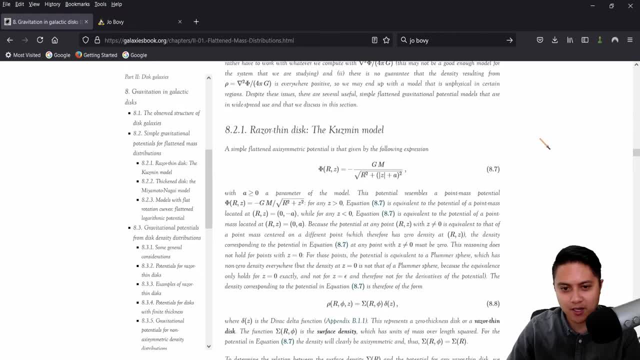 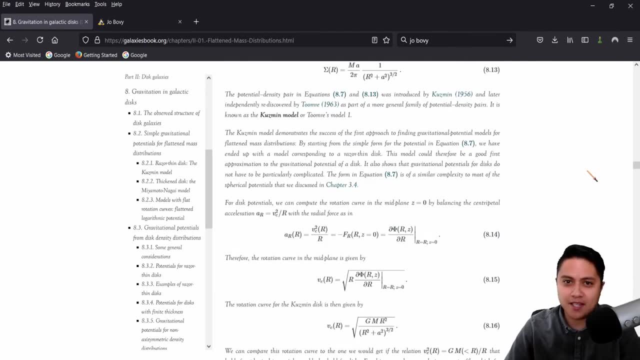 going in. I'm so for it. I'm looking forward to this one coming out. I'm looking forward to use this more in my own research when I need to reference things, And I think that's all I really have to say about this. I mean, this is just there's just too much to go through for one video. 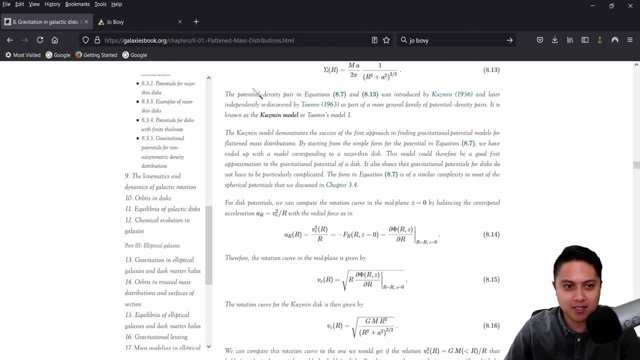 but if you're really interested, you can go ahead and hit the subscribe button. I'll see you in the next one. If you're interested, definitely check out galaxiesbookorg to learn the material yourself If you're really interested in galactic dynamics. I hope you found this video useful and insightful. 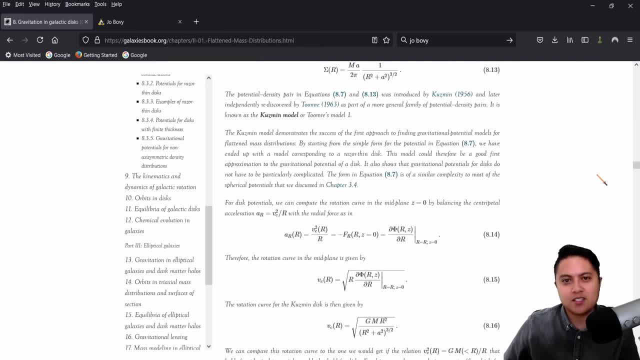 as to how important a book like this is to the field, And I hope you will come back for more videos relating to physics, astrophysics, astronomy and just my life as a PhD student in physics. So thank you for watching. I hope you enjoy the video and I will see you next time. Have a good day everyone.